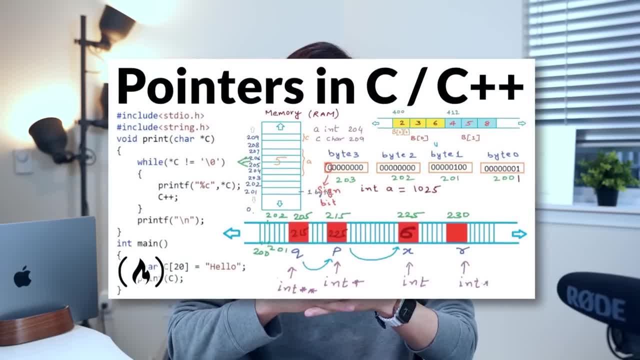 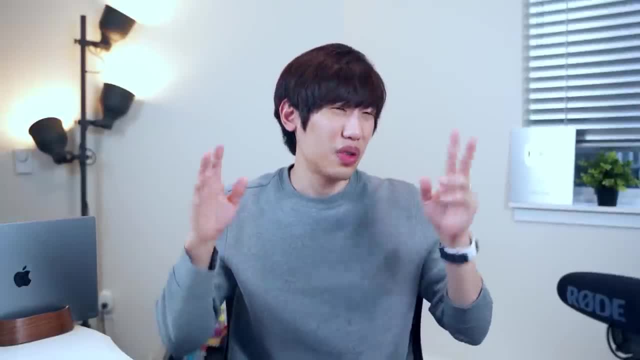 curve, with many beginners struggling with concepts like pointers and memory management. But again, you can learn more about C++ in the description of this video. If you want to learn more about C++, avoid them with Python. As a beginner coder, you should focus on how coding works. 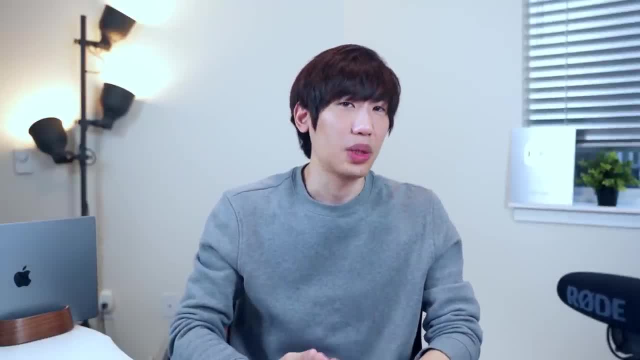 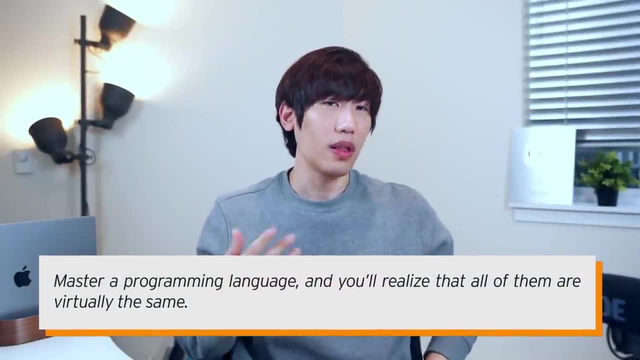 not how the language works. Don't make the mistake of learning another language prematurely either. Concentrate on becoming proficient with one first Master, a programming language, and you'll realize that all of them are virtually the same. The second reason I recommend Python is its popularity in the industry. 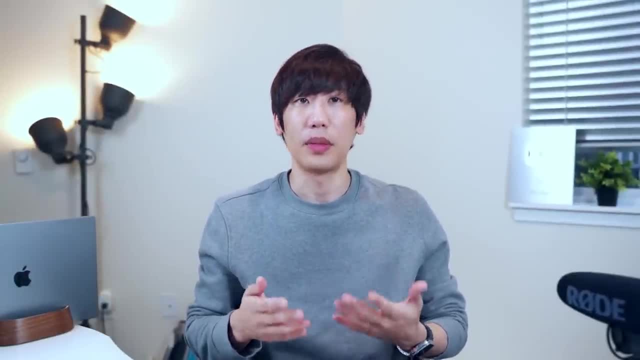 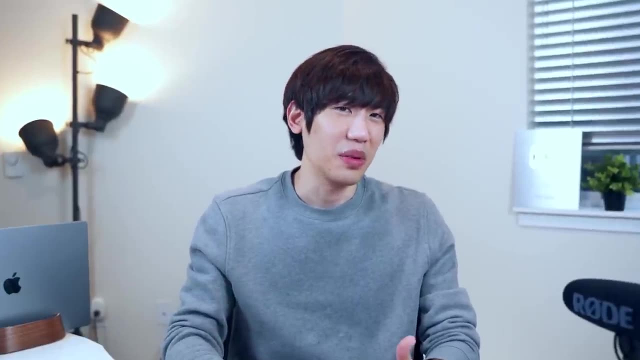 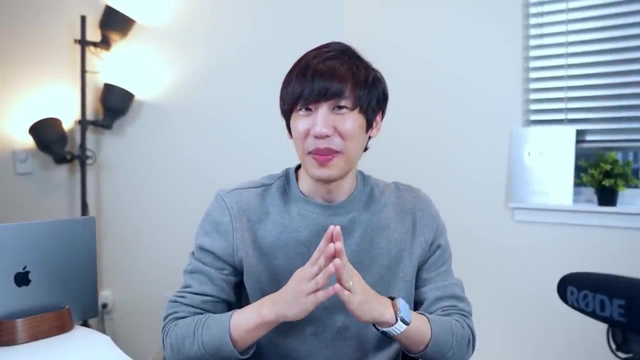 Its wide usage in various business sectors, such as web development, machine learning and data science, opens up multiple job opportunities. After all, if the programming language isn't practical, how will you get a job? right Now that we know Python is the right choice, let's discuss how to learn it. 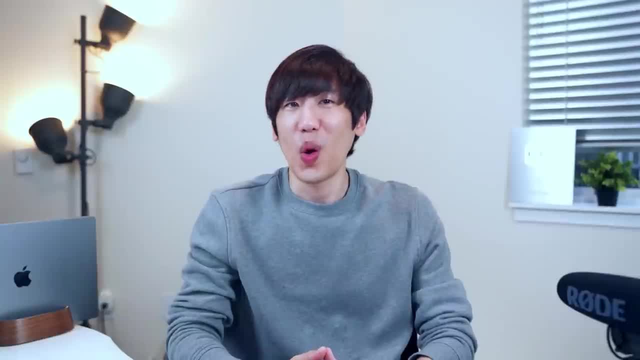 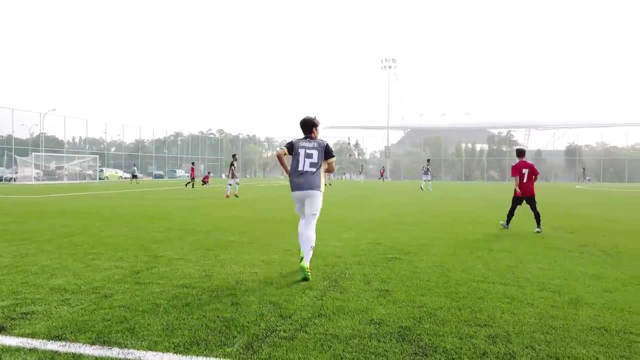 As I explained in how I would learn to code, the best way to learn to code is always to do it. Think of it this way: You get better at soccer by playing soccer and not watching someone else play Likewise. there's only so much you can learn just by watching videos and reading textbooks. 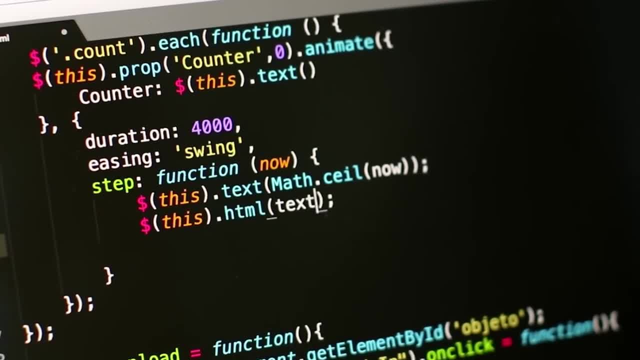 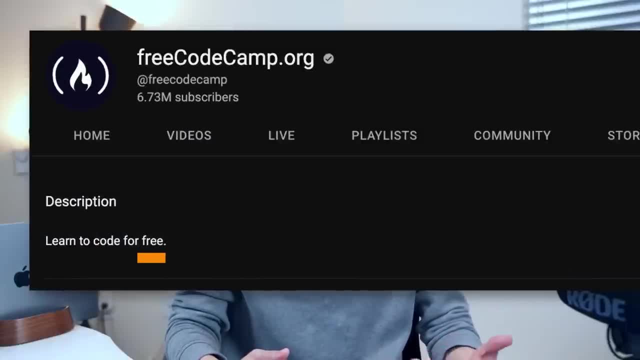 You must follow along, write the code yourself, do the exercises and so on. I recommend this YouTube channel, freecodecamporg. It's one of the best places 12 learn to code for free. Their courses are easy to follow and taught by the industry experts. 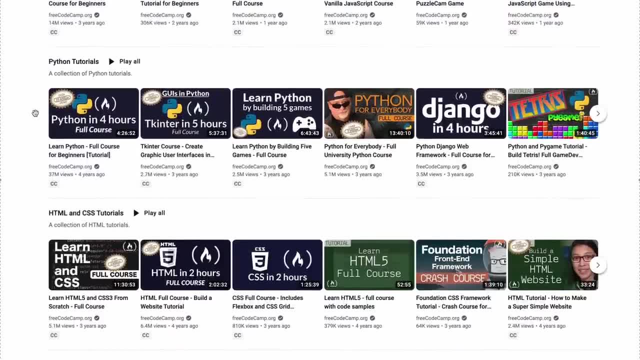 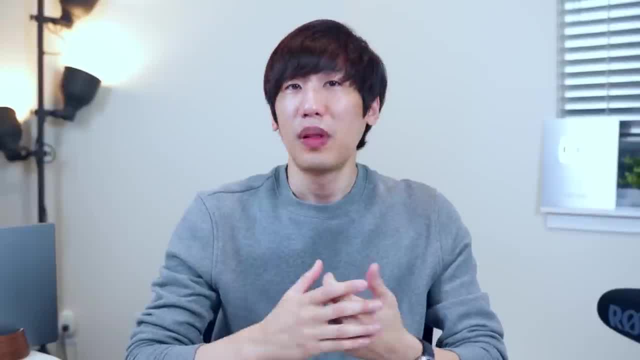 I learned many different languages and frameworks from their videos too. Start with their full course on Python for beginners. You can learn the fundamentals of Python without any prior coding experience. Once you've completed the tutorial, it's time to hone your skills by building projects. 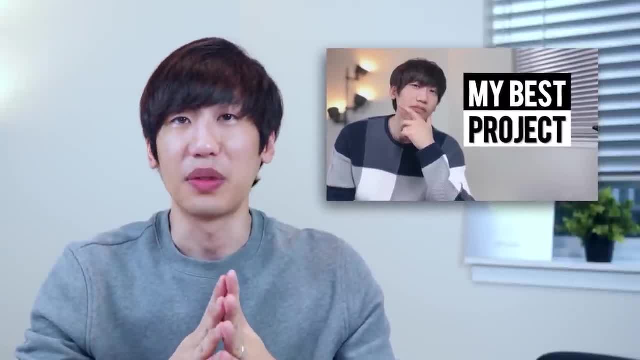 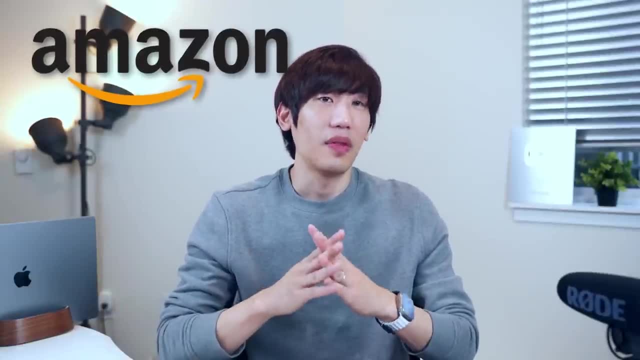 I already explained why this is essential in my past videos. I'll reiterate them briefly here. Number one: Growth. You'll learn significantly by doing so. Imagine building the mini Amazon, Facebook and Reddit. You'll begin to understand how they work at a high level. 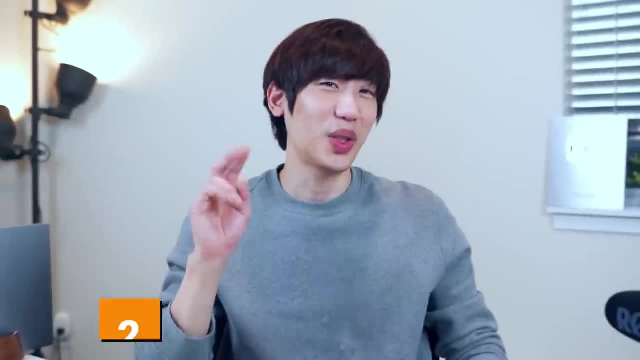 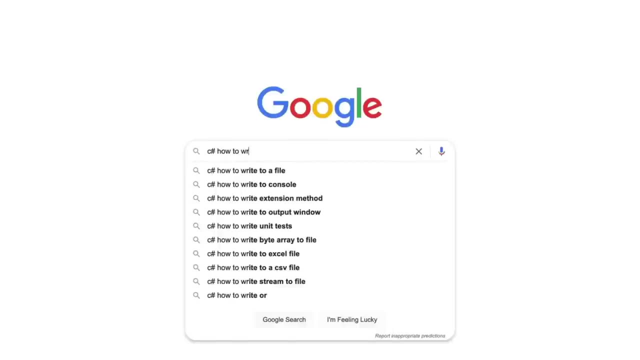 and be empowered to solve more challenging problems ahead. Number two: Experience. It'll introduce you to how software engineers work in the real world: Writing code, debugging, googling and, finally, copy and pasting. That's precisely what a day in the life of a software engineer looks like. 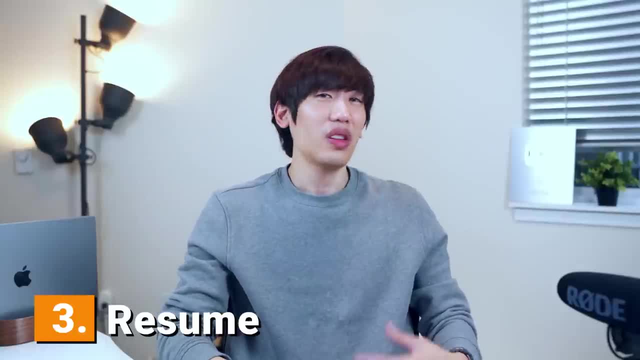 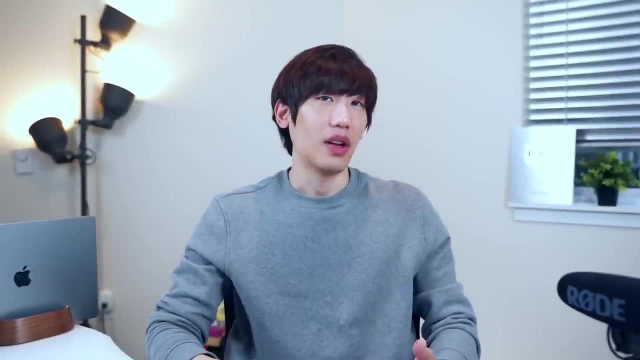 Minus working lying down. Number three Resume: By working on your projects, you'll automatically build your own portfolio. Put them on your resume with links to your Github or the website. For a detailed guide on how to craft an effective resume, check out this video. 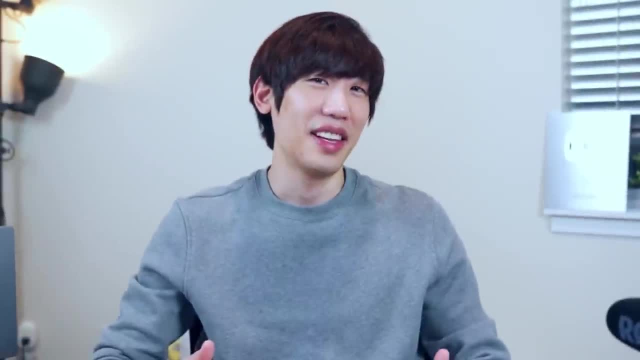 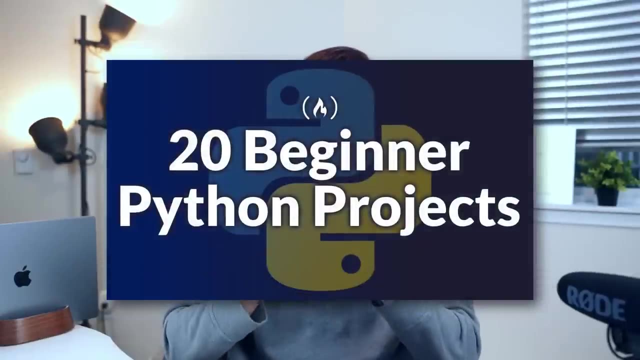 You can also download a copy of my resume from my website. Then the next big question is: what kind of project should you build? Again, learn with Free Code Camp. Start with the 20 beginner Python projects here. Follow along writing the code yourself until you fully understand. 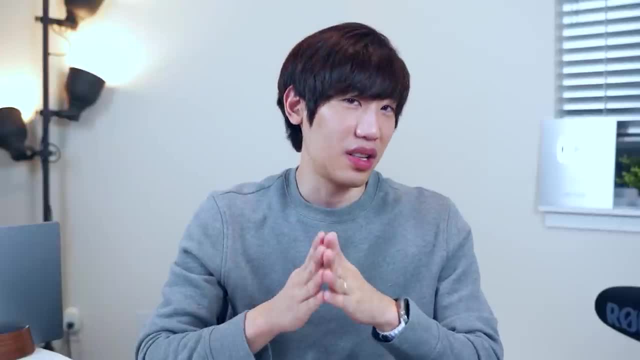 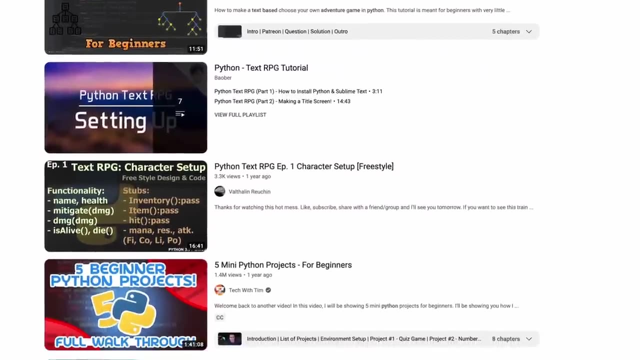 Once you've completed the course, it's time to build more complex stuff. You can add more features to the course, To the small projects you worked on earlier, Or make something fun like games, From a text RPG to Zelda-style games in Python. there are various free tutorials on YouTube. 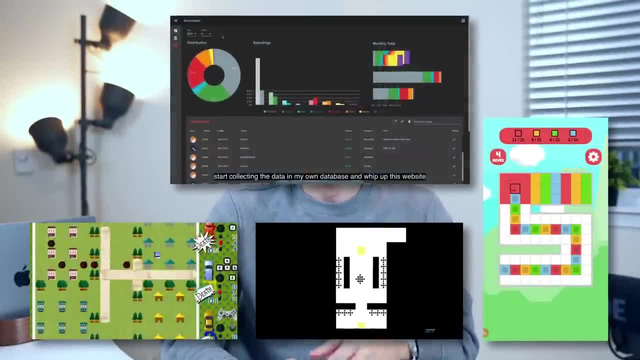 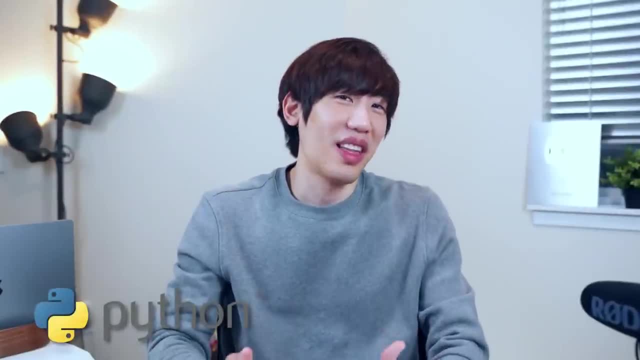 Personally, I made three games, including an award-winning one, and a personal finance website. For more project ideas, including how I built my website, check out this video Cool. You've learned Python, built projects and crafted a superb resume. 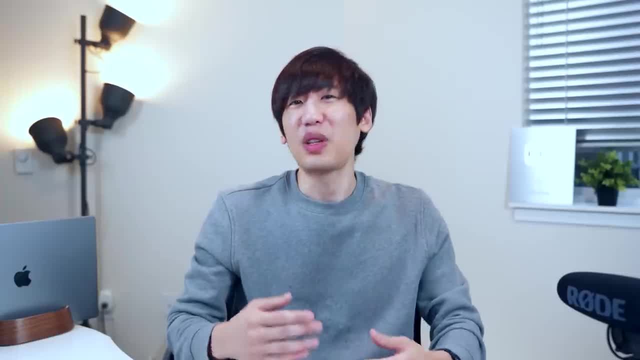 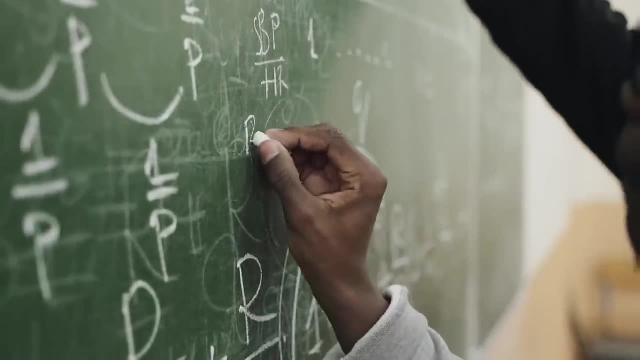 Should we apply for jobs right away? Wrong, Everything up to this point will help you land. what we call a coding in A coding interview is a technical challenge where a candidate is asked to solve a coding problem. Many companies, including Fang, love to play these games to evaluate you. 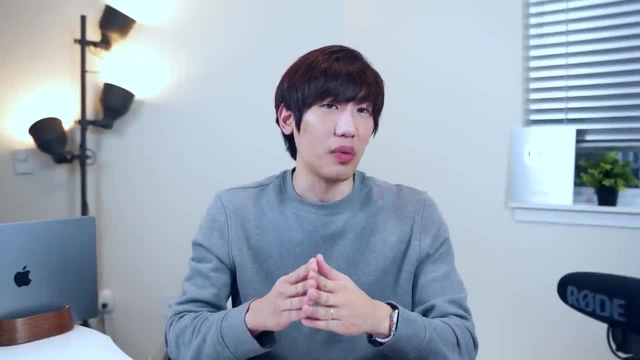 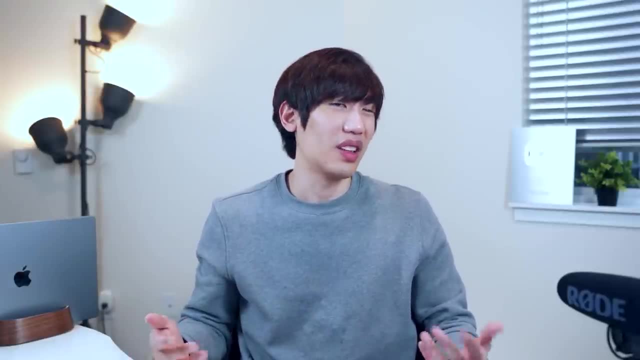 Some people neglect to prepare for them, arguing that coding interviews are irrelevant to your daily work. However, that's not a prudent strategy, as you'll have to play by this rule one way or another. Now then, how do you prepare for coding interviews? 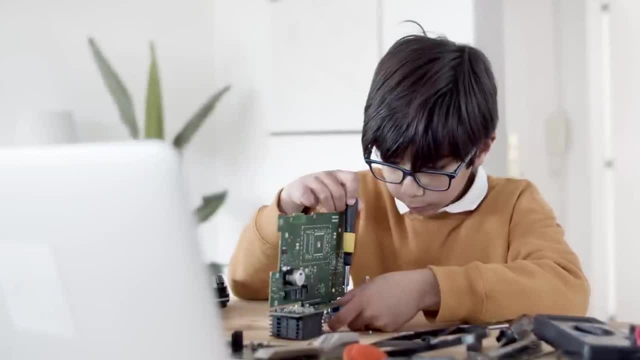 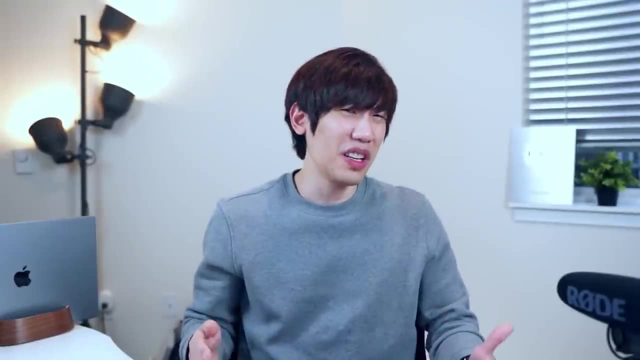 Study: DSA: Data Structures and Algorithms. Simply put, DSA is the fundamentals of computer science. Coding interviews are applications of its concepts. Where can you learn DSA for free? You guessed it: Free Code Camp. They have a complete Python course on Data Structures and Algorithms for beginners. 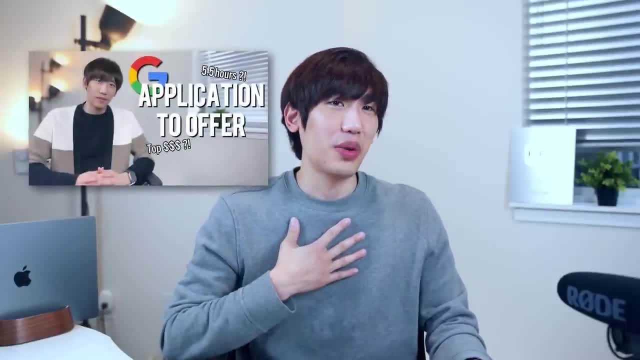 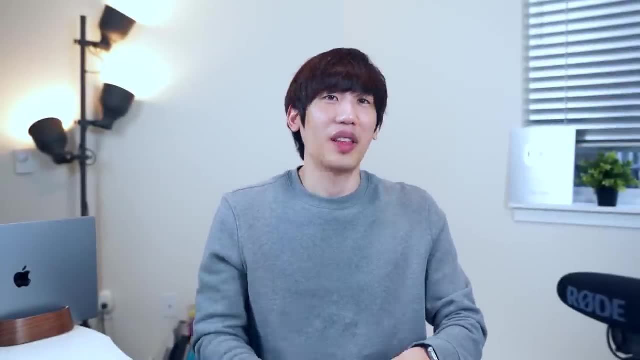 Having cracked many Fang interviews, including Google's, I can assure you that this video is everything you need to crack yours. Now that you've learned the concepts, it's time to put them into practice. The best platform to prepare for coding interviews is Leetcode. 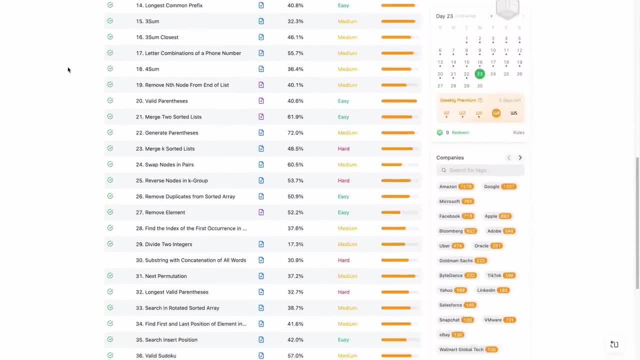 This is where all the software engineers, including industry professionals at Fang, come to sharpen their skills. The software engineers and engineers at Fang can provide help on the freelance process. Leetcode is a platform for you to learn a level of software and to try and change your life in a multiple way. 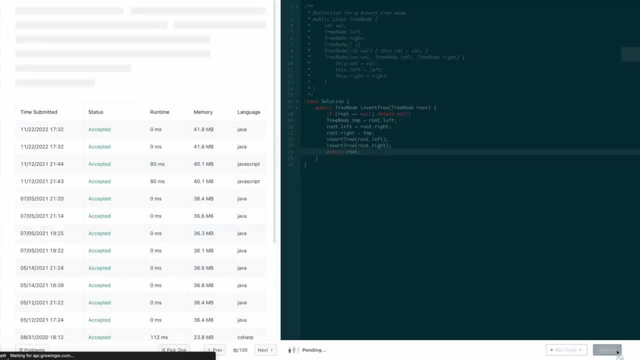 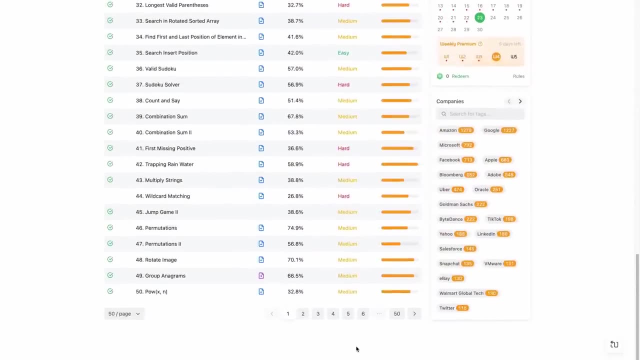 Leetcode is a platform for you to learn a lot of things. code is awesome because you can write code and test your solutions directly on their website. many of the problems in their database are real interview questions too. when you visit the code for the first time, the sheer number of problems can be daunting. i mean, there are nearly. 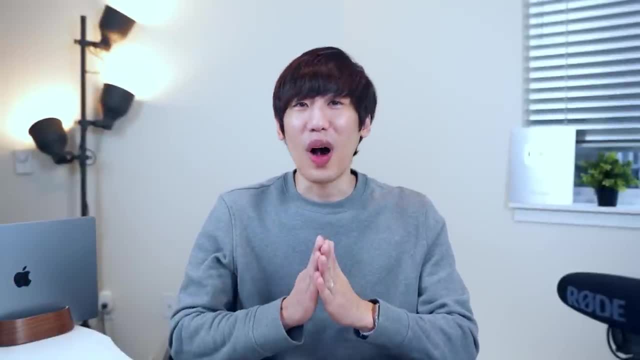 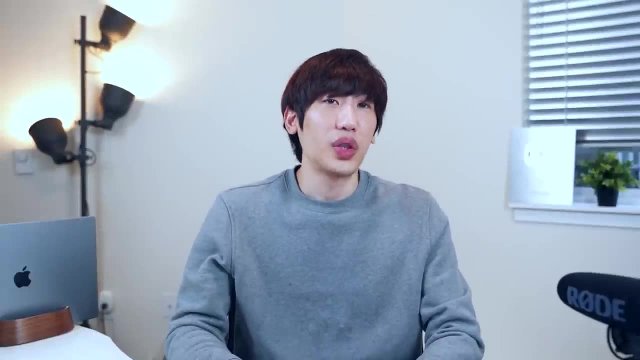 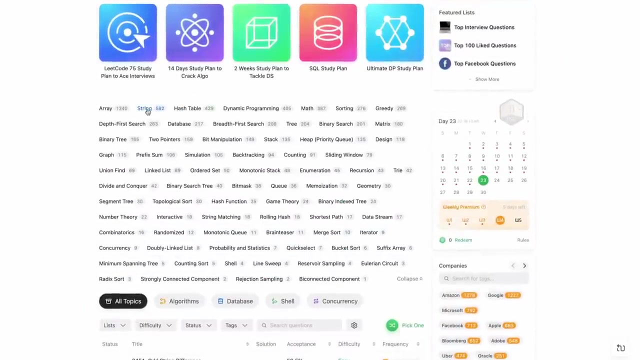 2500. it's overwhelming, i know, but that's why i created a video on how to use leetcode effectively to help you get started. refer to it for details, but i'll share the two don'ts from the video. one: don't solve random problems. instead grind the questions on the same topic. 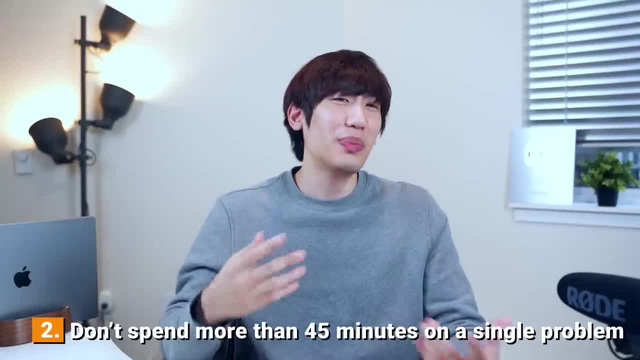 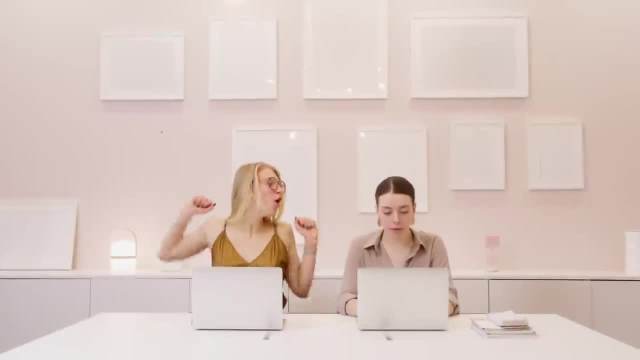 until you get a click on the patterns. two: don't spend more than 45 minutes on a single problem. if you can't figure it out, look up the solution, however, learn from it, then come back to the same question. until you can solve it without help, you're ready to apply for the jobs if you can. 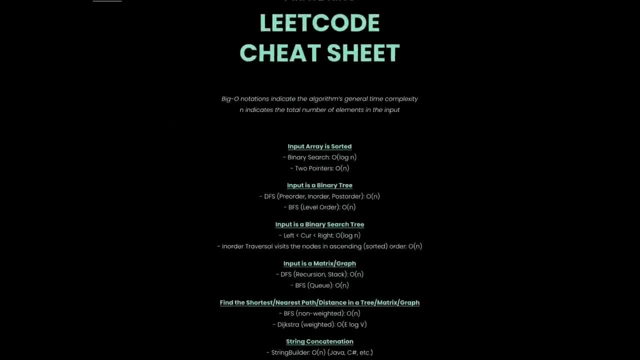 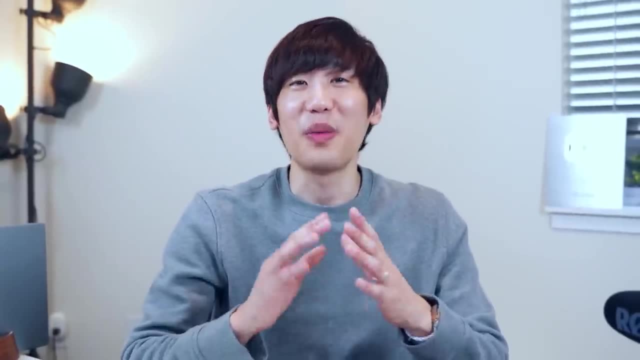 solve a meeting problem in 45 minutes. to help your study, i created a leeko cheat sheet, along with the study guide and helpful resources on my website for free. now let's take a look at the. oh. by the way, i put together a curriculum, or everything we discussed so far, on my website. 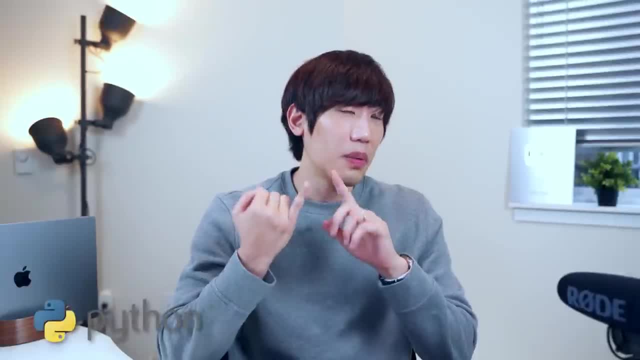 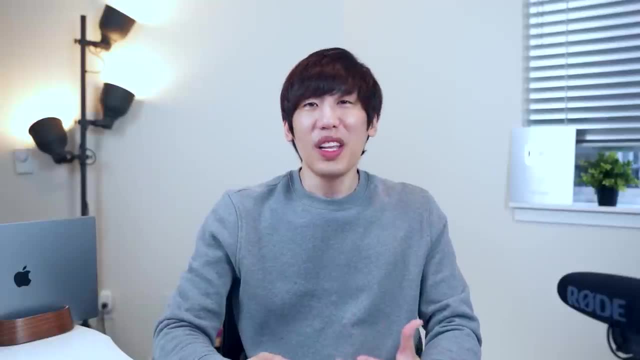 for free. just follow the pages in order. in summary, learn python, build projects, study dsa and finally solve leetcode. if you do the math, that's nearly 20 hours of video time on free code camp tutorials alone, which is pretty good, to be honest. university computer science lectures are generally 45 hours. 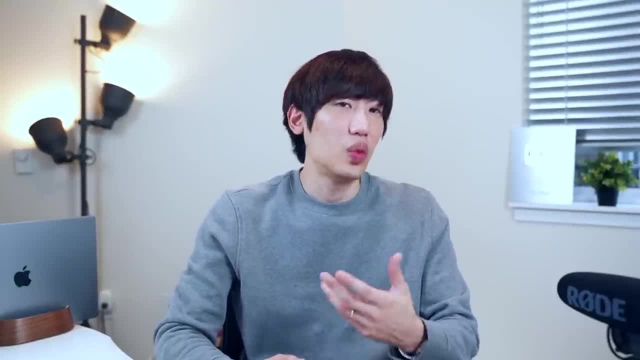 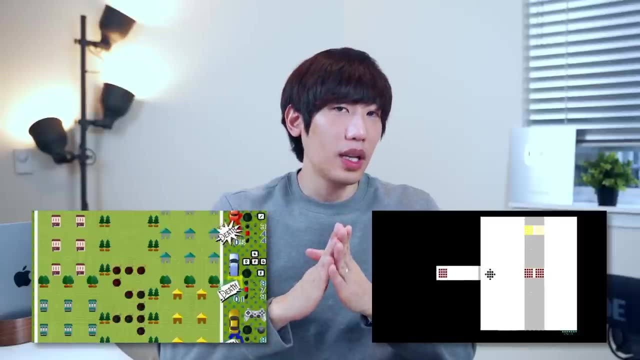 of class time per semester. you're learning the essentials in just 20.. in addition to the tutorials, i recommend you build at least two high quality projects, spending about 40 to 60 hours each. once you have your project and resume ready, move on to leetcode. there's no fixed timeline for leet. 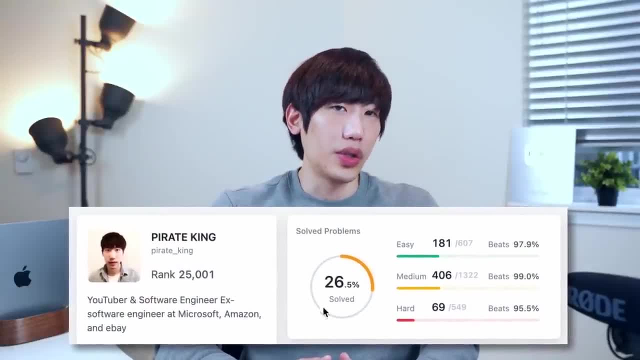 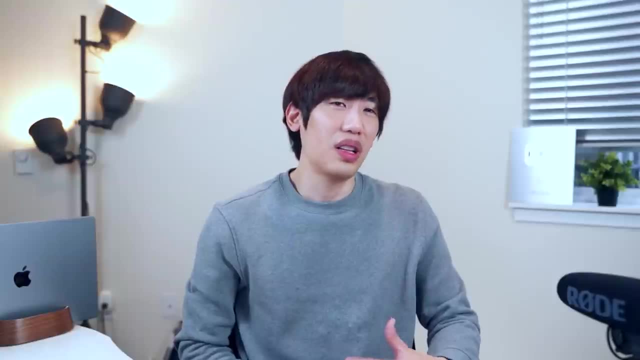 code, but i suggest you solve at least 150 questions before actively applying for jobs. all right, we discussed the fastest way to become a software engineer for free. if you're still unconfident and prefer an affordable alternative, consider giving springboards coding bootcamp a try. you can get a thousand dollar discount off their career-friendly software engineers program if you're still in a competitive situation with you. all right, we discussed the fastest way to become a software engineer for free. if you're still unconfident and prefer an affordable alternative, consider giving springboards coding